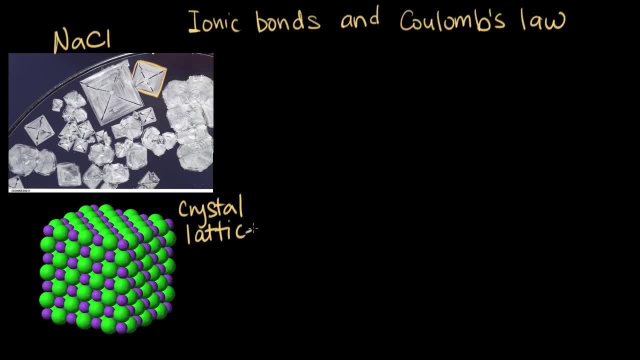 And you can look at the crystal lattice and get information about how the different ions are arranged in these solids. So the way that the ions are arranged determines a lot of things about the properties of these compounds, So these ionic bonds and how the ions are arranged. 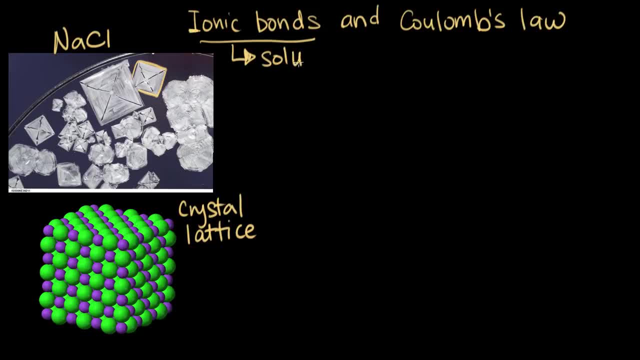 tell us a lot about the solubility of the compound Solubility And other properties like melting or boiling points, And it even can be related back to things like how hard a particular ionic solid is. So the ionic bonds here in sodium chloride. 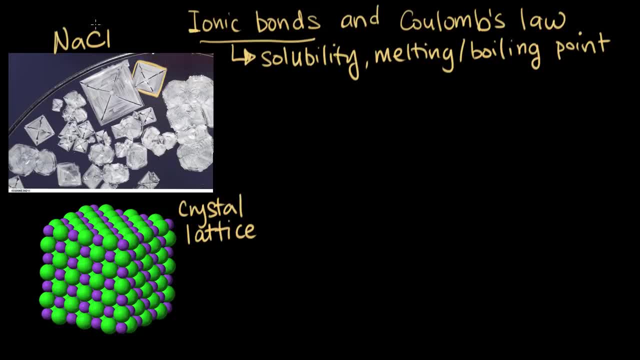 are the ones that hold together our sodium ions and our chloride ions. So our sodium plus and our chloride minus. And the strength of an ionic bond is related to the electrostatic force, The electrostatic force between them, And I'm going to abbreviate the electrostatic force. 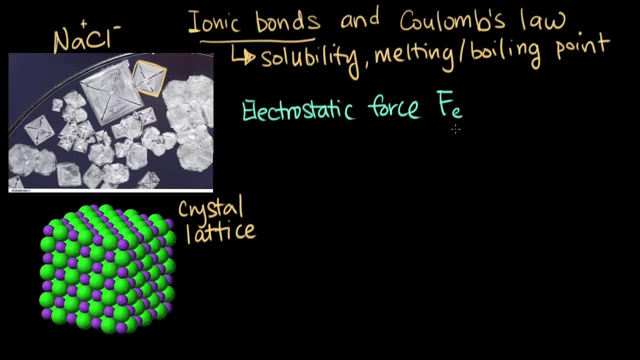 as F, subscript E. So this is the force between two charged species And it's equal to some constant K times the two charges that are interacting Divided by the distance between the two charges squared. So here Q1 and Q2 are the charges. 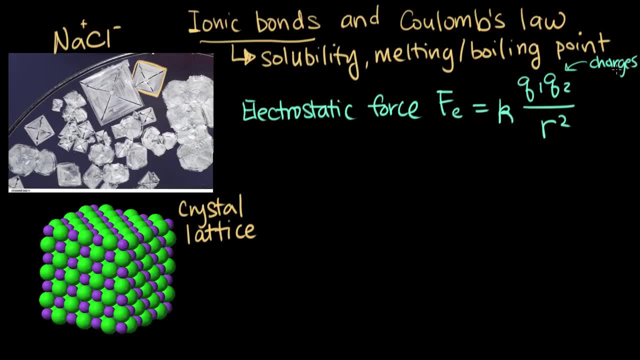 And in the case of sodium chloride, for example, Q1 and Q2 would be. Q1 might be 1 plus from our sodium ion And Q2 might be 1 minus from our chloride ion, And we could also just switch those two. 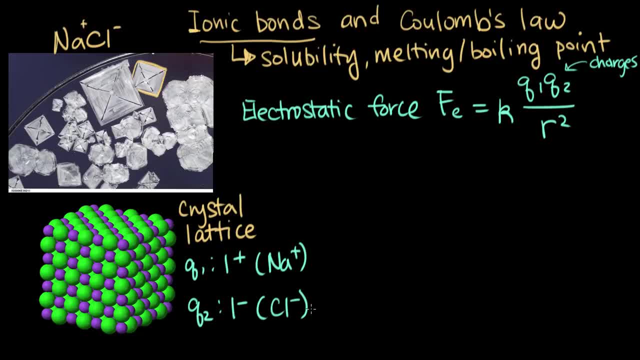 We could say Chloride is Q1 and sodium is Q2. And that wouldn't change what we get from this equation. And then R2: here is the distance between the ions, And we usually approximate it as saying it's the sum of the ionic radii. 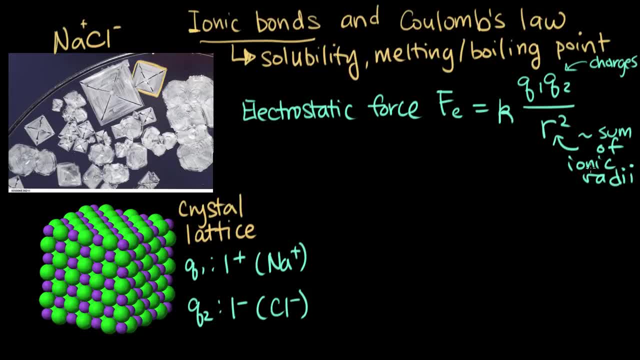 for the two ions we're looking at. So we can use Coulomb's Law here to explain some properties that are related to the strengths of ionic bonds, And so the example we're going to go through today is going to be that of melting point. 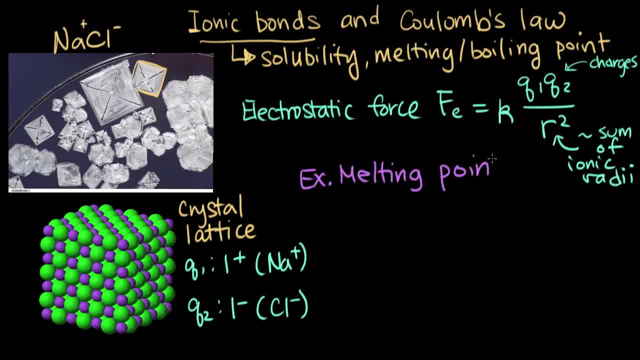 So we're going to look at some melting point trends and try to relate them to the different variables in Coulomb's Law. So the first thing we'll look at, the first two compounds we'll compare are sodium fluoride and magnesium oxide. Sodium fluoride has a melting point. 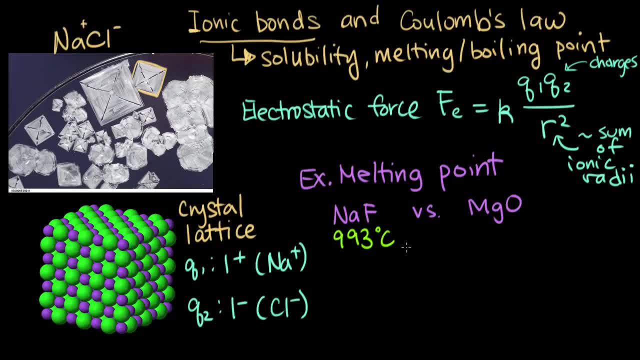 of 993 degrees Celsius, And magnesium oxide has a melting point of 2,852 degrees Celsius. The other information we know about these two compounds: if you look up the ionic radii, it turns out that sodium fluoride- the distance between the ions- 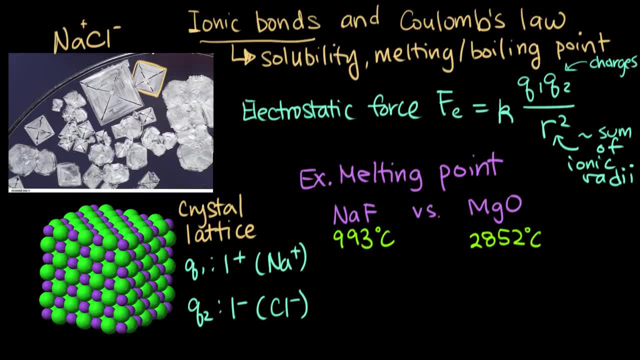 is about the same as magnesium oxide. They're not exactly the same, but they're pretty close. So if we were to say that R is approximately the same for these two, then we can explain the difference in melting points using the charges. 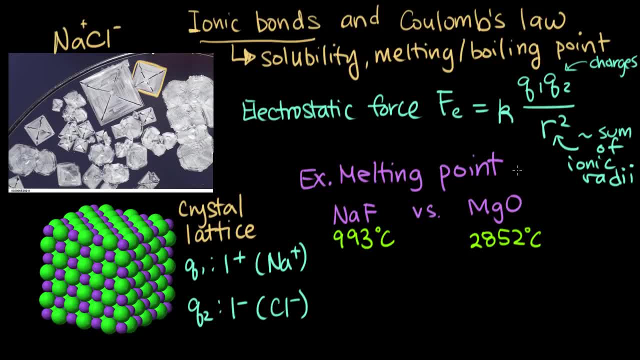 Since melting point is a measure of basically how much energy do you need to add to these compounds to break apart your ions, we would expect melting point to go up, to increase. as Fe increases. As the force between the ions increases, we would expect to have to add more energy. 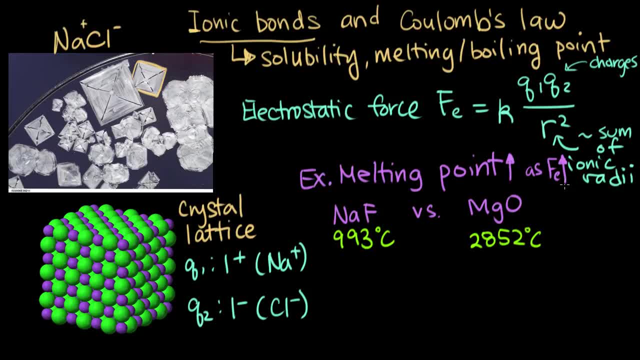 to break those ions apart And we can see that in our first example, Magnesium oxide, if we look at the charges on the ions, magnesium is two plus and oxide is two minus. In sodium, fluoride, sodium is one plus and fluoride is one minus. 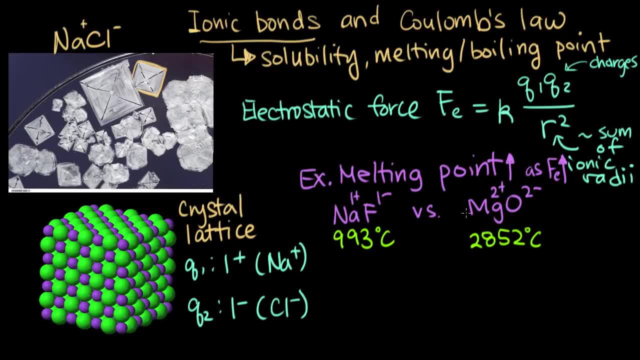 So we would expect, assuming that R is about the same, Q1 times Q2 is four times bigger in magnesium oxide versus sodium fluoride. So Q1 and Q2, product of Q1 and Q2, is higher for magnesium oxide, and that's why we would expect. the melting point to be higher. We can also look at sodium chloride versus sodium fluoride And in this case let's look at- well, I don't know, maybe this is kind of artificial- The melting point of sodium chloride is 801 degrees Celsius.